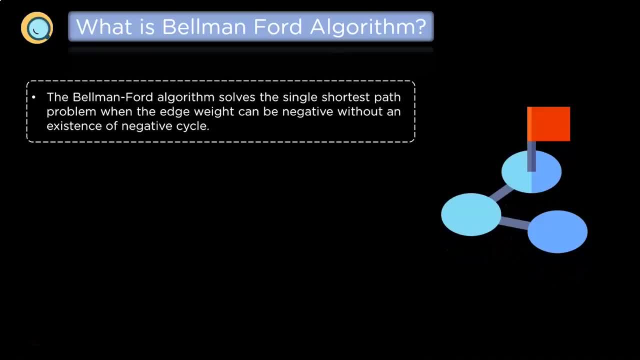 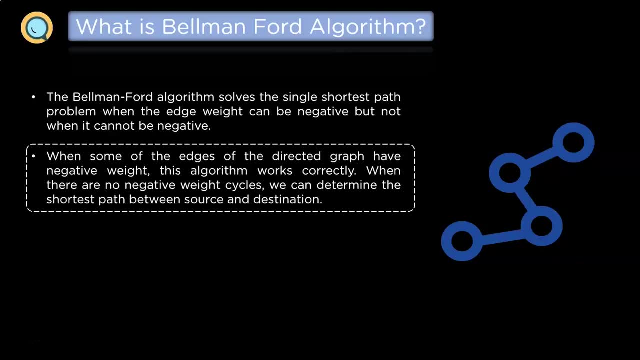 can be negative without a negative cycle. When some of the edges of the dedicated graph have negative weight, the algorithm works correctly. When some of the edges of the directed graph have negative weight, this algorithm works correctly. When there are no negative weight cycles, we can determine the 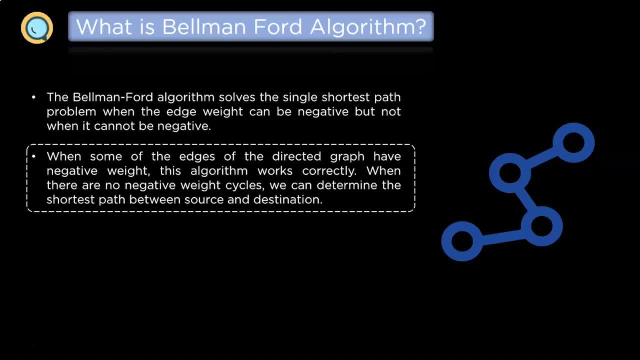 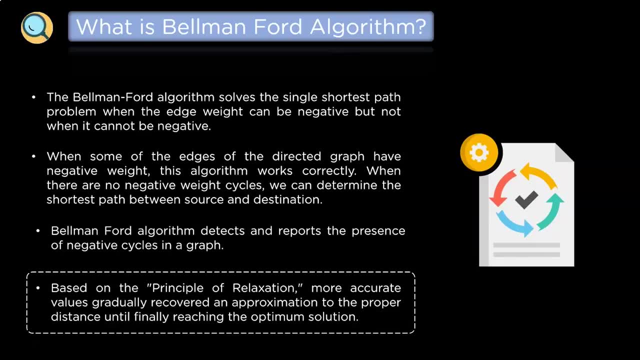 shortest path between source and destination. The Bellman-Ford algorithm detects and reports the presence of negative edge weight cycles in a graph Based on the principle of relaxation, more accurate values gradually recovered, an approximation to the proper distance until finally reached the optimum solution. After understanding what exactly is Bellman-Ford algorithm, we 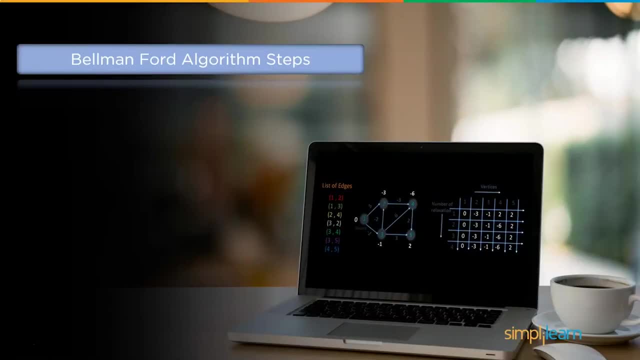 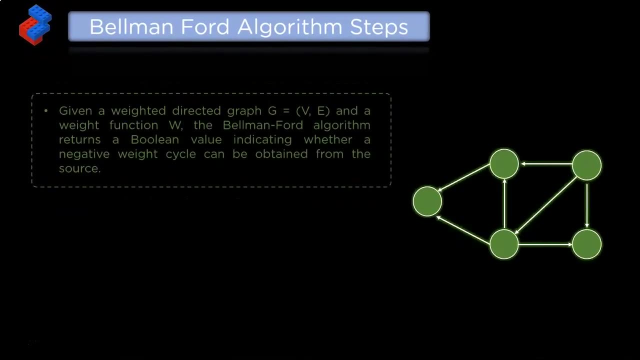 will now look into some of the steps followed by the Bellman-Ford algorithm, But let us look at one scenario. Given a weighted directed graph, G is equals to V comma e, that is, vertices and edges, and V comma e, that is vertices and edges, and 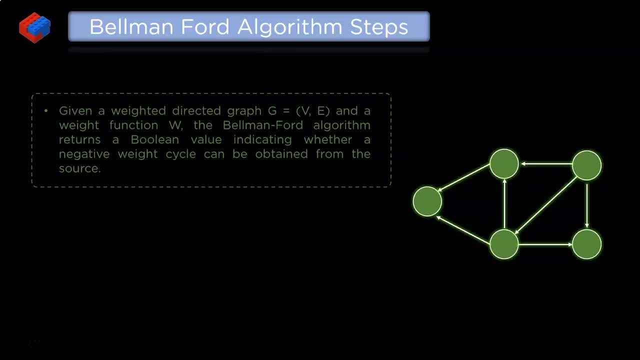 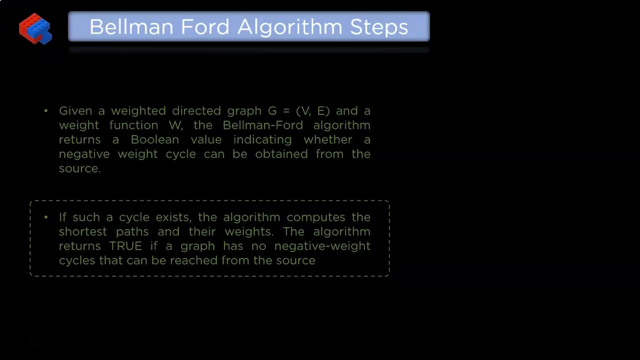 a weight function W. the Bellman-Ford algorithm returns a Boolean value indicating whether a negative weight cycle can be obtained from the source or not. If such a cycle exists, the algorithm computes the shortest paths and their weights. The algorithm returns true if a graph has no negative weight cycles. that 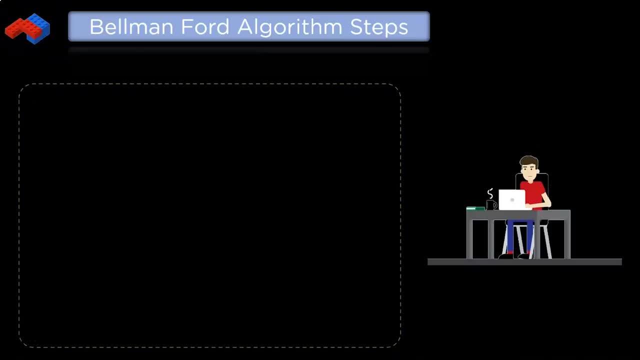 can be reached from the source. Let us start with the Bellman-Ford steps for one-dimensional calibration to see how it works. Set the distance values of nodes to infinity, except the source node. In the first step we must repeat the relaxation step V minus 1 times. 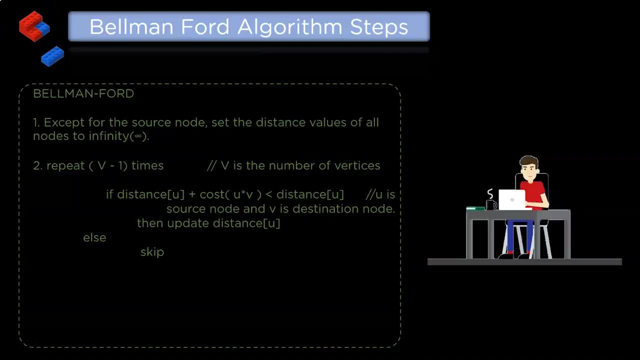 where V is the number of vertices. So if we have an edge from U to V, where U is the source node and V is the destination node, then V will be updated with a new distance value of the distance of U plus the cost of the edge Uv. at this point, 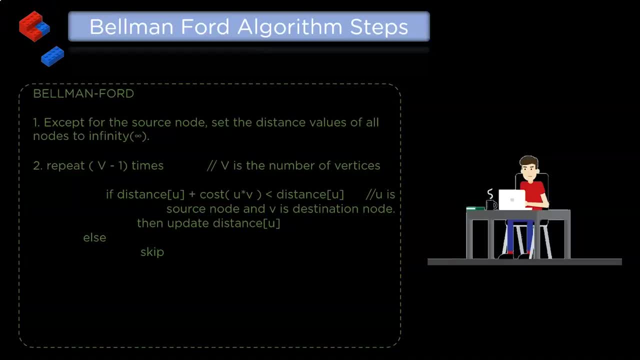 is less than the distance of V node. Otherwise we will not update it and we will skip it. All vertices should be relaxed once more. We have a negative edge weight cycle if we find a new, shortest distance value. Otherwise, we do not have a negative edge weight cycle. 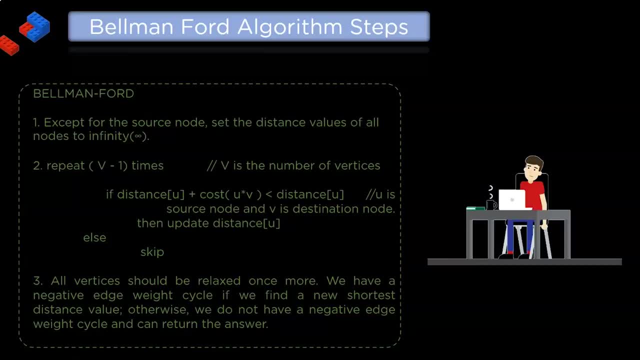 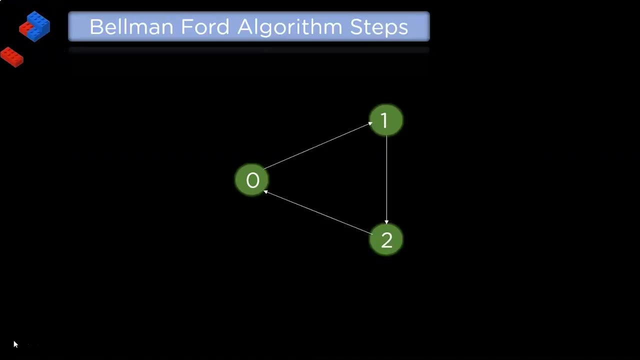 and can return to the answer in the last step. We have heard that the Bellman force algorithm is used to detect a negative edge weight cycle in the graph for a long time. Let us see how the Bellman force algorithm detects a negative edge weight cycle in the graph. 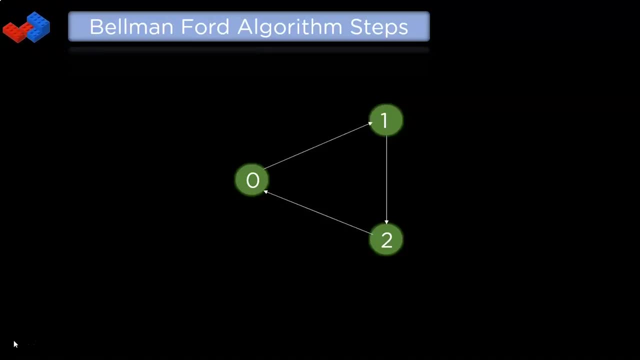 Let us assume that we have a graph with three vertices, with initial value as infinity as the weight of the graph. Because this graph has three vertices, we will relax it V minus 1 times, that is, 2 times In the first time of relaxation. 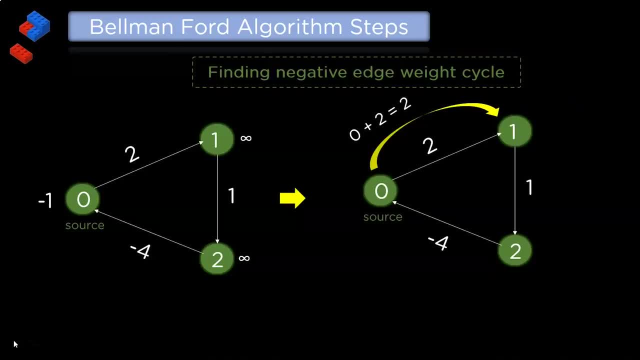 the weight from 0 to 1 is 2.. So the cost of 0 to 1 will be 0 plus 2, which is equal to 2.. So because 2 is less than infinity, we will replace infinity by 2.. Now, from 1 to 2, the cost will be 2 plus 1. 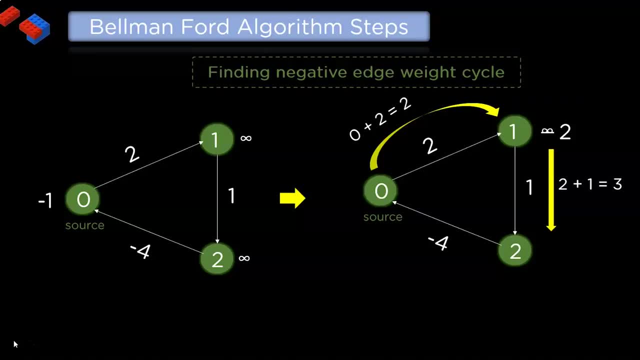 which is 3, which is less than infinity, So that we will replace by infinity by 3.. After that, we have got 2 to 0. The cost will be 3 plus minus 4, which is equal to minus 1, and as we know that, 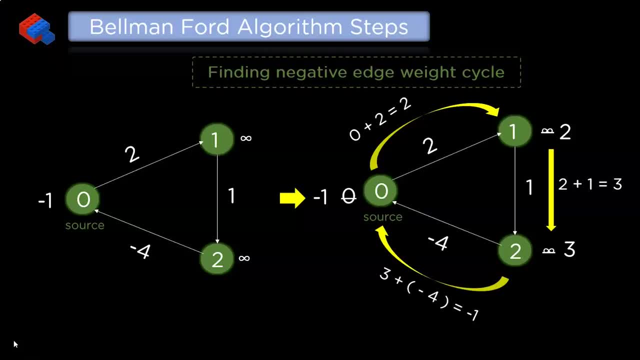 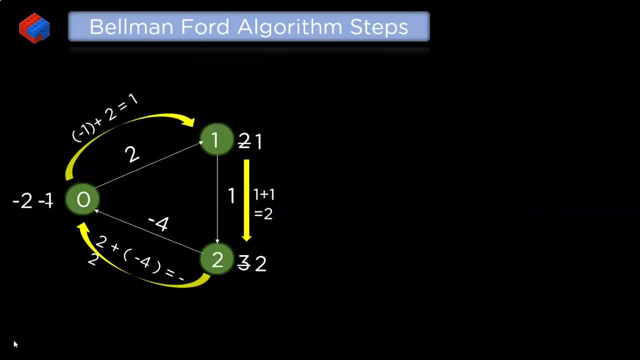 minus 1 is less than 0, we will replace it 2.. In the second time of relaxation, the weight from 0 to 1 is 2.. So the cost from 0 to 1 will be minus 1 plus 2, which is equal to 1, and 1 is less. 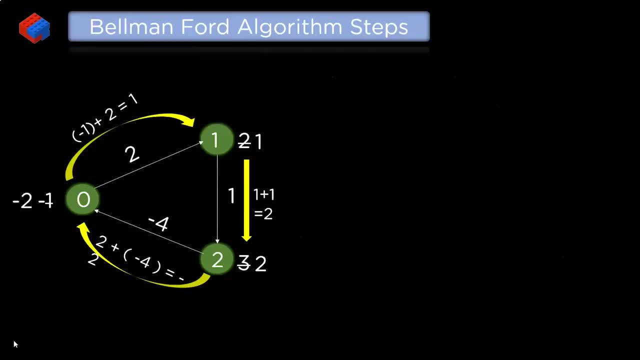 than 2.. So we will replace it by 2.. So the cost from 0 to 1 will be minus 1 plus 2, which is equal to minus 1.. Now, from 0 to 1, we have the weight as 1.. The cost will be 1 plus 1, which will be: 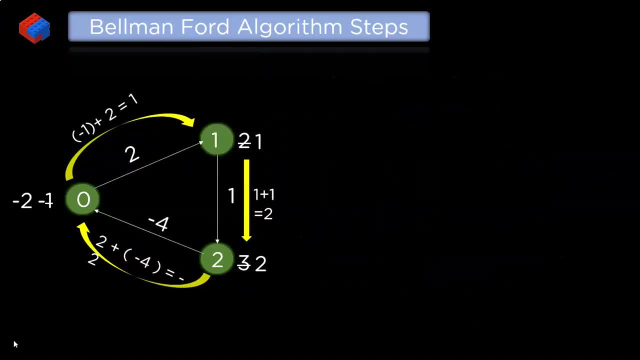 equals to 2 and we know that it is less than 3.. So we will replace 3 by 2.. Finally, from 2 to 0, we have weight as minus 4.. So the cost will be 2 plus minus 4, which is equals to minus 2, and. 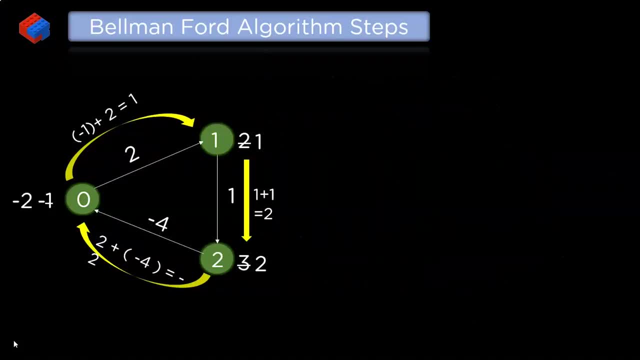 minus 2 is less than minus 1.. So we will replace minus 1 by minus 2.. We have finished the first two times of relaxation, So let us try the third time. In the third time of relaxation we have the weight from 0 to 1 as 2. 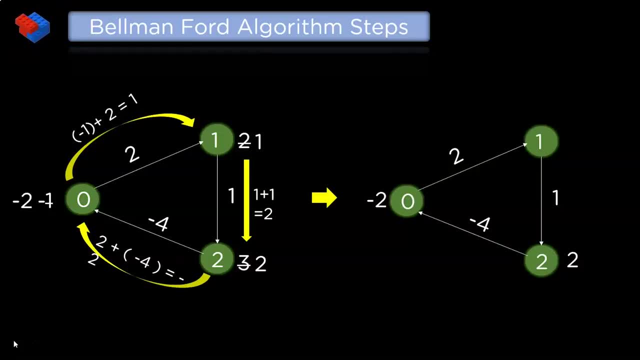 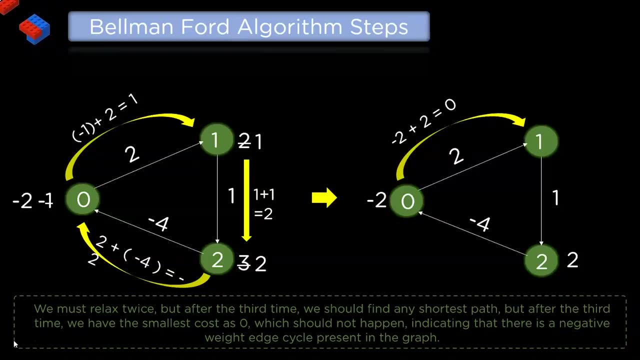 and the cost will be minus 2 plus 2, which is equals to 0, and 0 is less than 1.. So we will replace 1 by 0.. So after performing the third time, we have minimum distance as 0.. 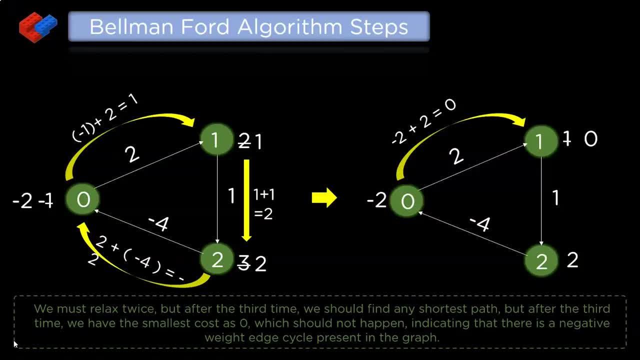 Which should not happen, because we only had to relax it twice. We must relax twice, But after the third time we should find the shortest path. But after the third time we have the smallest cost as 0, which should not happen, indicating that there is a negative weight edge cycle. 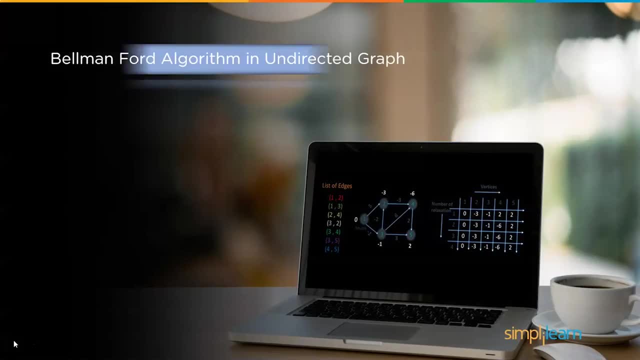 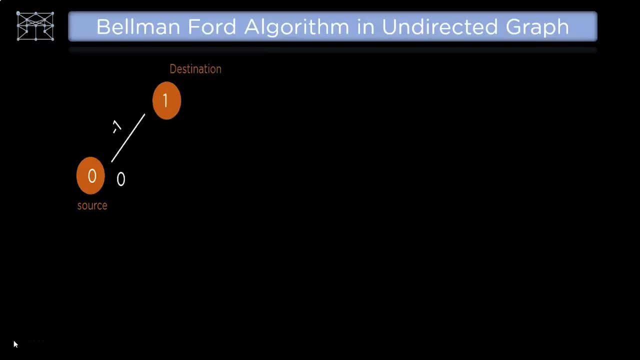 present in the graph. Next we will see how the Bellman-Ford algorithm works on an undirected graph. We will learn this through an example. Here we have a graph of two vertices: 0 and 1.. So when we go from undirected edge 0 to 1, the cost will be calculated as 0 plus minus 1. 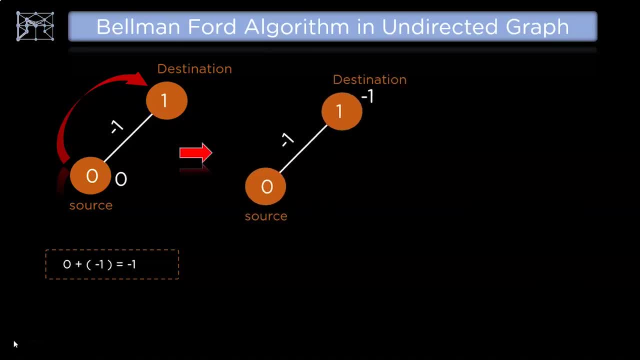 which is equals to minus 1.. Now, from edge 1 to 0, the edge will be minus 1 plus minus 1, which is equivalent to minus 2.. Now again, if we want to calculate the minimum cost, it will be minus 2 plus minus 1, that is minus. 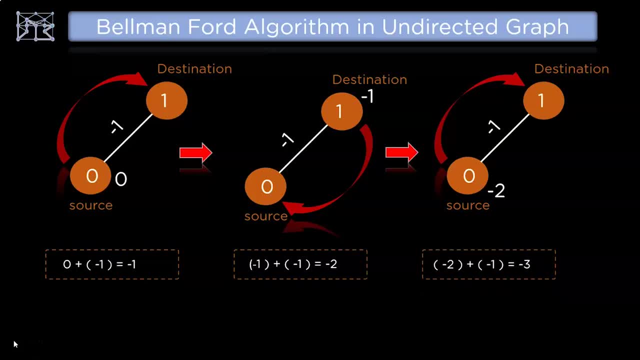 3 and this will be turned as an infinite loop. So here we come with two points. The Bellman-Ford algorithm works only if all the edges are undirected graph are positive. If an undirected graph has any negative edges, the Bellman-Ford algorithms fail to find a path For better. 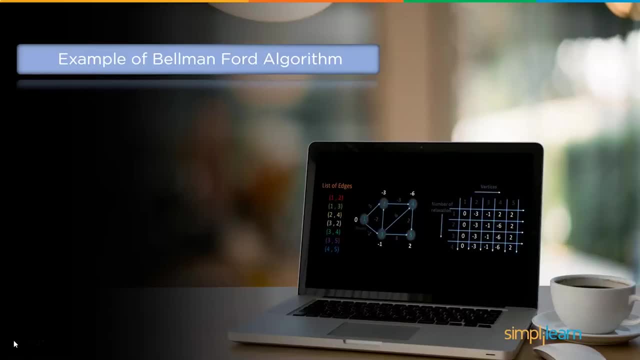 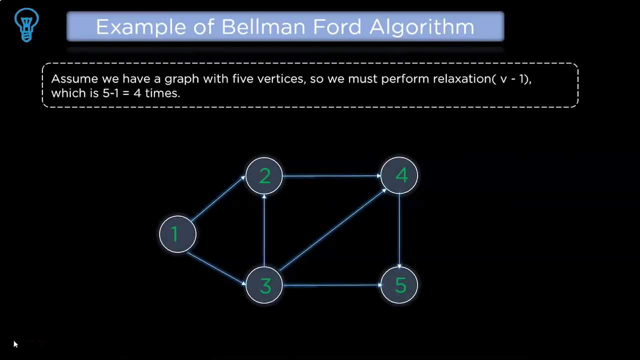 understanding. let us look at an example for Bellman-Ford algorithm. Assume that we have a graph with five vertices, So we must perform relaxation v minus 1 times that is. 5 minus 1 times that is 4.. Following that is a table in which we will update the minimum cost of the edges. 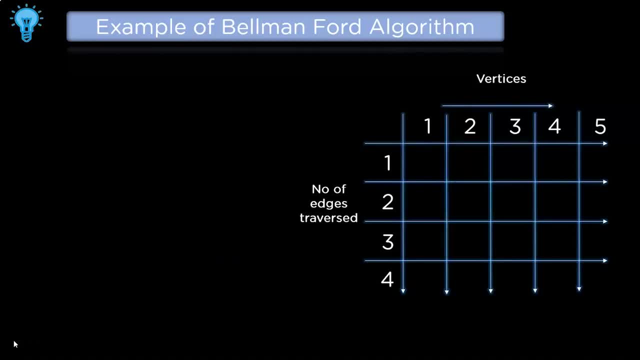 of this graph, where the column is for vertices and edges is for the number of edges traversed. Next we have a list of edges that are 1, 2, 3,, 4,, 5,, 6,, 7,, 8,, 9,, 10,, 11,, 12,, 12,, 13,, 13,, 14,. 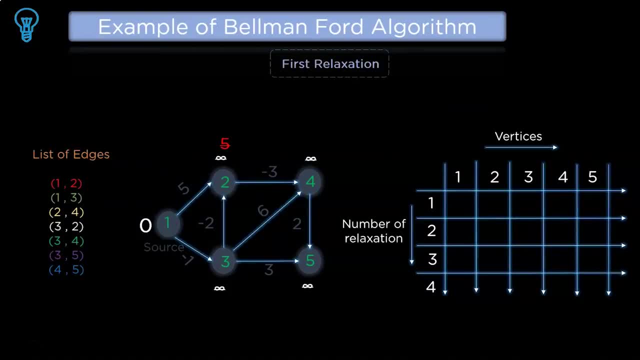 15, and 20, and finally, 4 to 5.. From 1 to 2 edge, the cost will be 0 plus 5, which is equal to 5, which is less than infinity, So that we will replace it with 5.. From 1 to 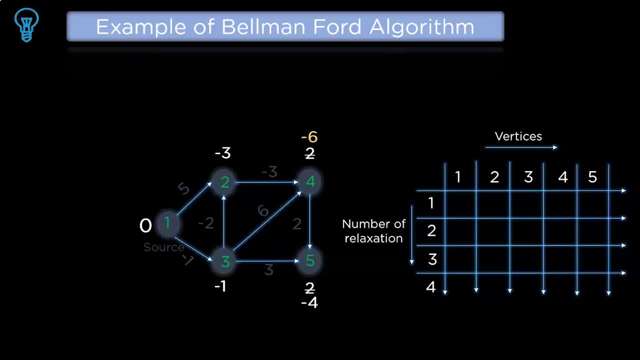 3 edge, the cost will be 0 plus minus 1, which is also less than infinity. So that will be replaced by minus 1.. Now, from 2 to 4 edge, we have the weight as minus 3.. 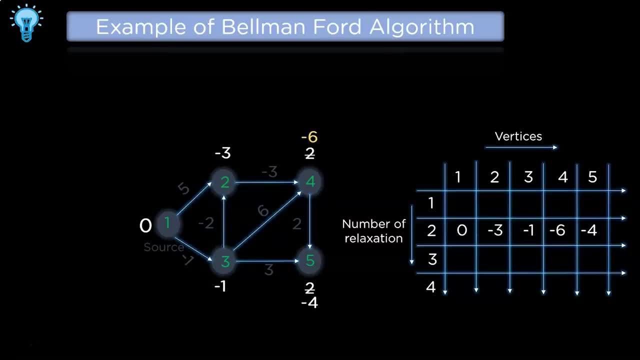 So the cost will be 5 plus minus 3, which is equals to 2.. And 2 is less than infinity, So we will replace it with 2.. From 3 to 2, we have the weight of minus 2.. 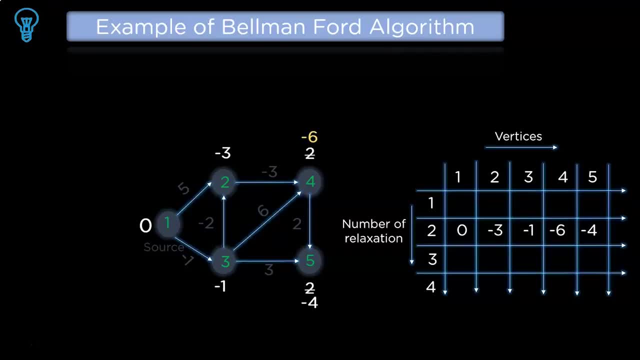 So the cost will be minus 1 plus minus 2, which is calculated as minus 3.. And minus 3 is less than 5.. So we will replace with minus 3.. Now, from 3 to 4, we have weight as 6.. 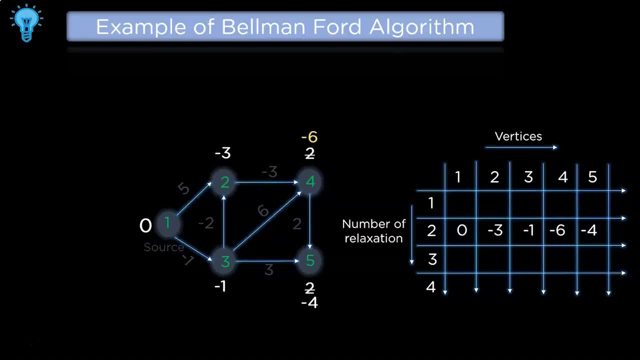 So the cost will be minus 1 plus 6, which will be calculated as 5.. But 5 is greater than 2. So we will not replace it Now. we have an edge of 3 to 5, where the weight is 3.. 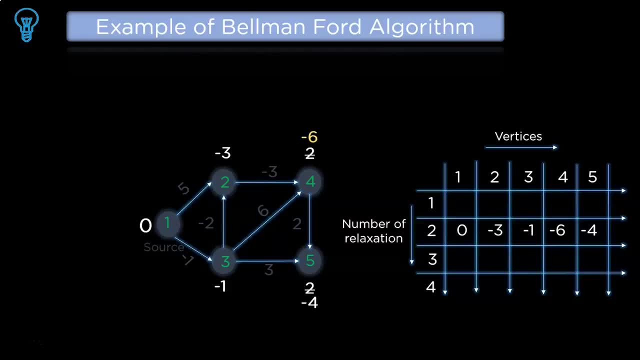 And the cost is calculated as minus 1 plus 3, which is 2.. And 2 is less than infinity. Finally, we have an edge of 4 to 5., Where the weight is 2. And the cost is calculated as 2 plus 2,, which is 4.. 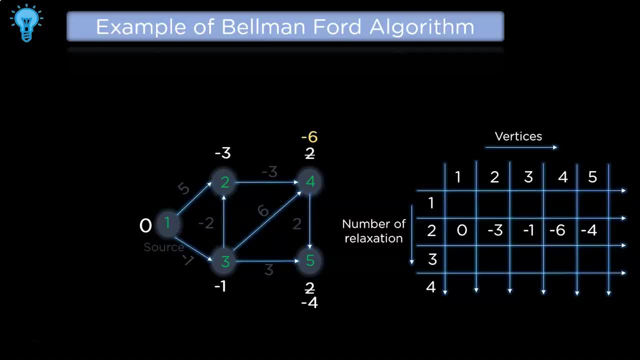 But 4 is greater than 2.. So we are not going to replace it. So in the table of the first relaxation we will now update all the vertices with minimum cost. Now let us move into second relaxation. From 1 to 2 edge, the cost is 0 plus 5, which is equals to 5, greater than minus 3.. 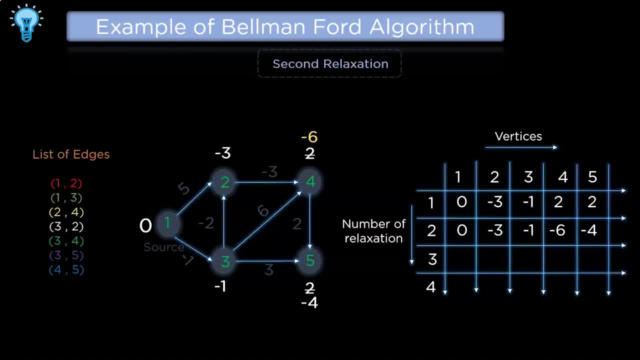 So we will not replace it. From 1 to 3 edge the cost is 0.. Plus minus 1, which is equals to minus 1, but we already have minus 1 as vertex number 3. So we will not update it. 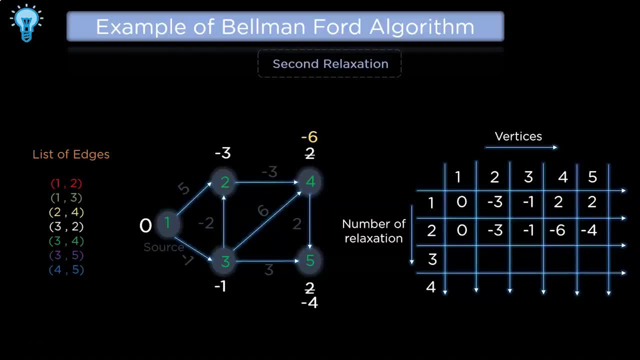 Now we weigh minus 3 from the 2 to 4 edge, So the cost is minus 3 plus minus 3, which is equals to minus 6.. And minus 6 is less than 2.. So we will replace it by minus 6.. 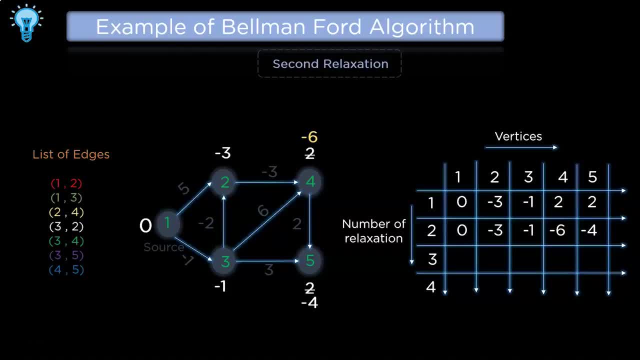 From 3 to 2, we have the weight of minus 3.. So the cost will be minus 1 plus minus 2, which is equals to minus 3.. And minus 3 is already there, So we won't update it. 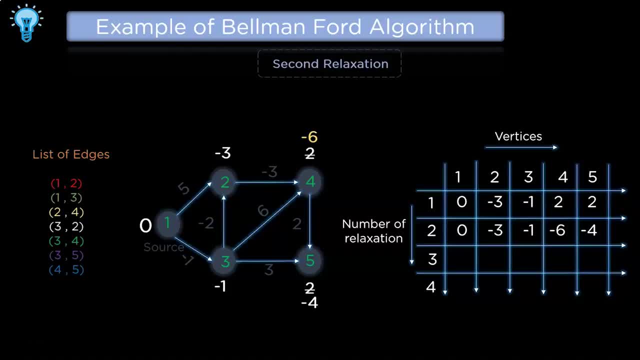 Now that we weigh 6 from 3 to 4, the cost will be minus 1 plus 6,, which is calculated as 5.. But 5 is greater than minus 6. So we will not be replacing it. 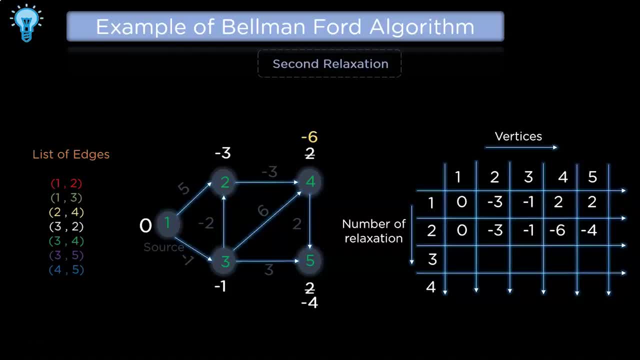 Now we have 3 to 5 edge, where the weight is 3. And the cost is calculated as minus 1 plus 3, which is equals to 2.. And 2 is already there, So we won't update it. 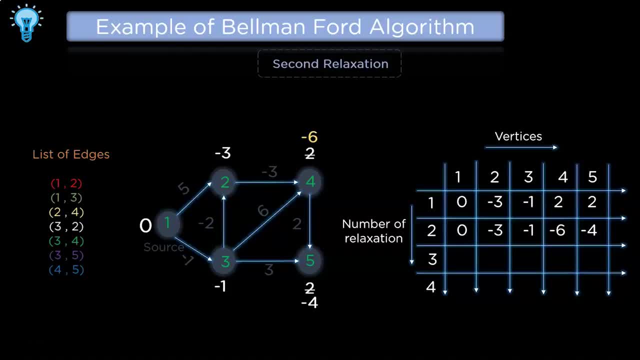 Finally, we have a 4 to 5 edge, where the weight is 2, and the cost is calculated as minus 6 plus 2,, which is equals to minus 4.. And minus 4 is less than 2.. 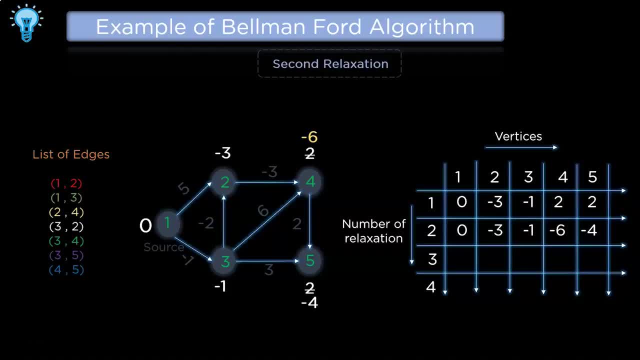 So we will replace minus 4 by 2.. So in the table of second relaxation we will update all the values. Now let us move to third relaxation stage. From edge 1 to 2, the cost is 0 plus 5,, which equals 5,, which is greater than minus 3.. 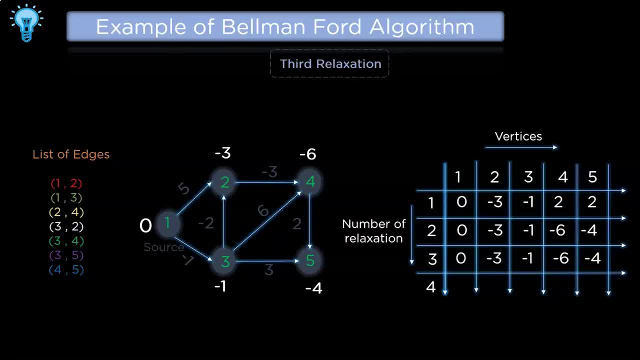 So we will not replace it. From the edge 1 to 3,, the weight is minus 1, and the cost is estimated as 0 plus minus 1, which equals minus 1.. But we already have minus 1 as vertex number 3.. 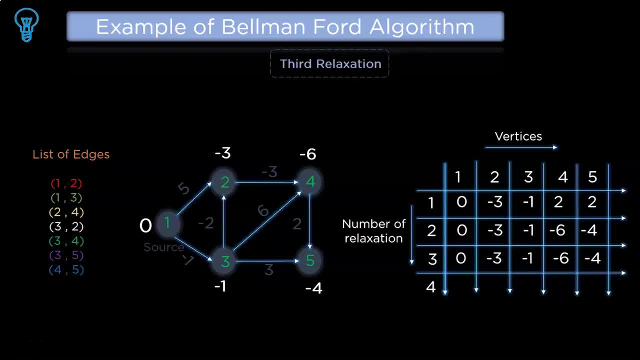 So we will not update it. Now. we have weight, So we will update minus 3 from the edge 2 to 4.. So the cost is minus 3 plus minus 3, which equals to minus 6.. 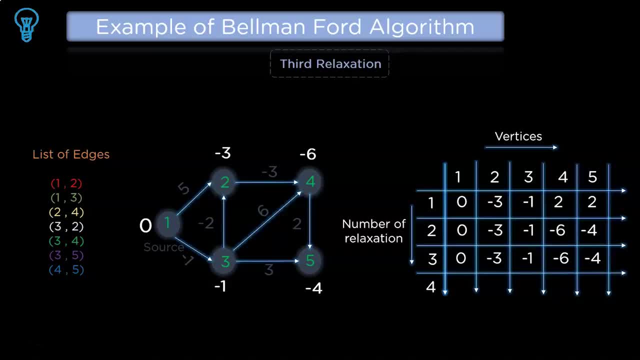 And minus 6 is already there, So we will not update it From 3 to 2, we have the weight as minus 2.. So the cost will be minus 1 plus minus 2,, which equals to minus 3.. 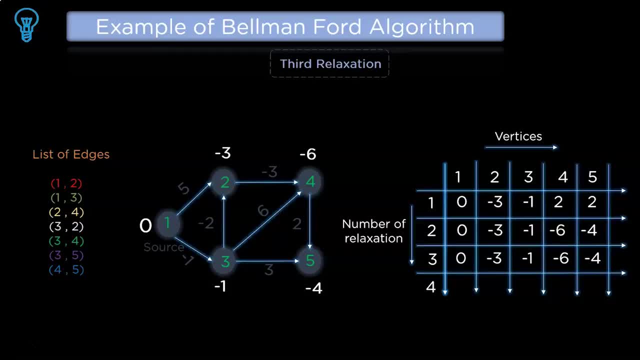 And minus 3 is already there, So we won't update it. Now that we weigh 6 from 3 to 4 edge: Now that we weigh 6 from 3 to 4 edge, the cost will be minus 1 plus 6, which is calculated as 5.. 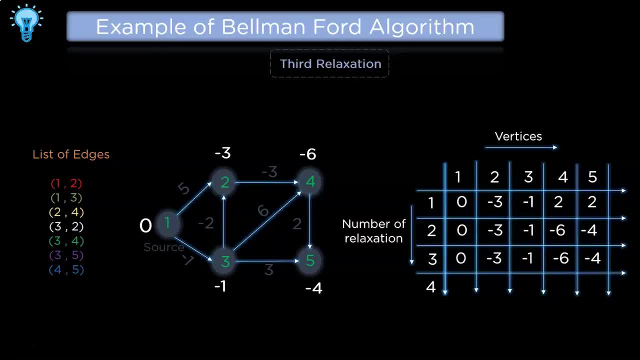 the cost will be minus 1 plus 6, which is calculated as 5.. but the value of 5 is greater than minus 6.. but the value of 5 is greater than minus 6.. So we will not replace it. 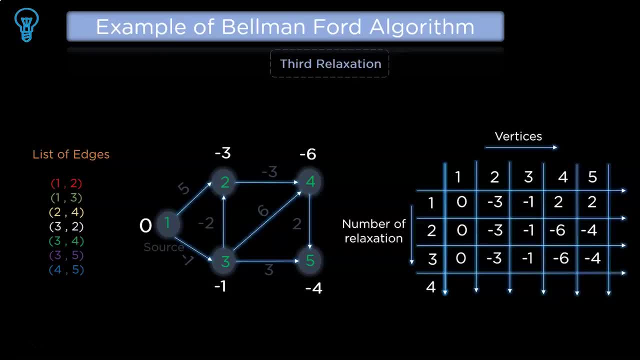 Now we have the edge 3 to 5,. Now we have the edge 3 to 5, with the weight as 3, and the cost is calculated as minus 1 plus 3,, which equals to 2.. And 2 is already there. 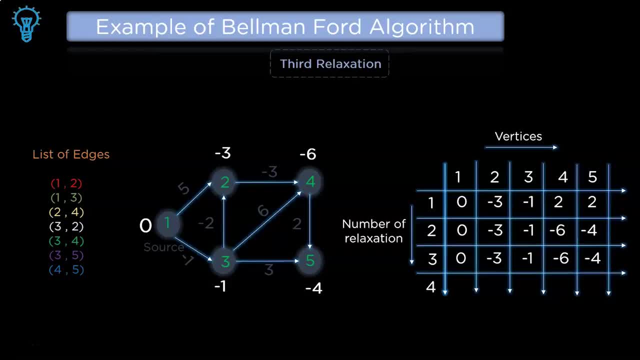 So we won't update it. Finally we have a 4 to 5 edge. Finally we have a 4 to 5 edge. the weight is 2 and the cost is calculated as minus 6 plus 2, and it is minus 4 and minus. 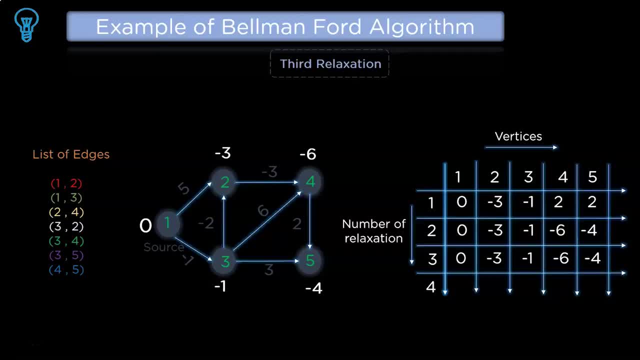 4 is already there, so we will not do anything. So in the table of third relaxation we will now update all the vertices with minimum cost. As we can see, we got the exact minimum cost for the third relaxation as we did for the second, which means we will get the actual minimum cost for the fourth time of relaxation. 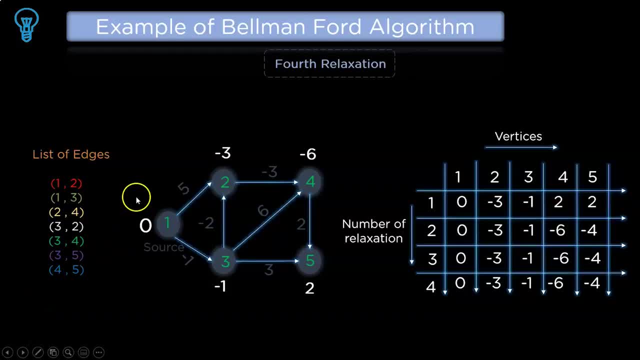 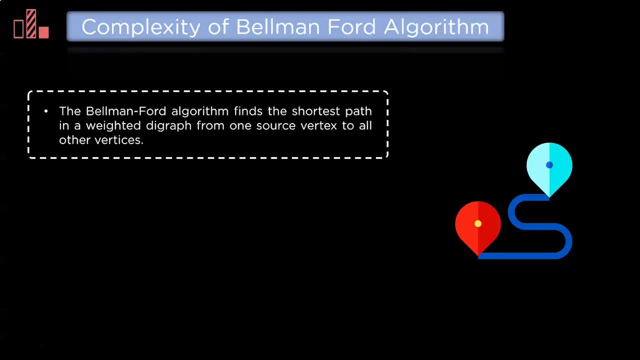 and now we have calculated the minimum cost of all the edges. Following that, we will examine the complexity of Bellman-Ford's algorithm. The Bellman-Ford algorithm finds the shortest path in a weighted diagraph from one source vertex to all the vertices. 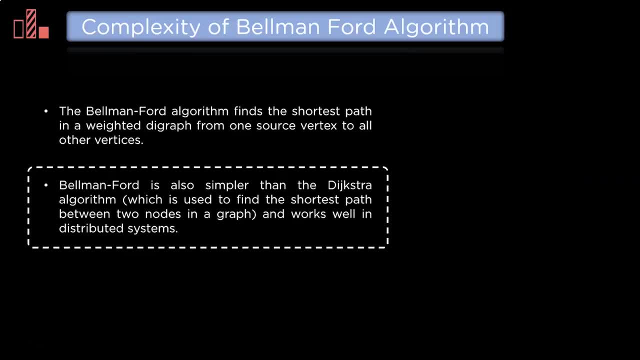 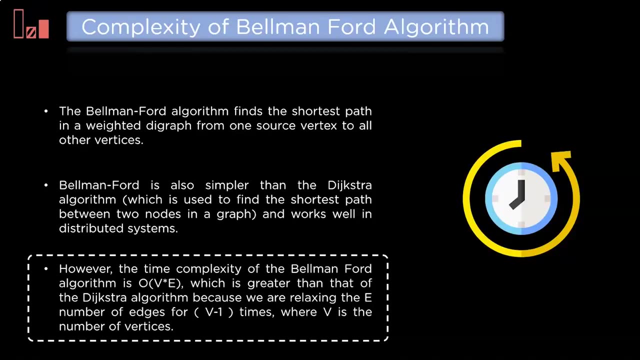 Bellman-Ford is more straightforward than the Dijkstra's algorithm used to find the shortest path between two nodes in a graph and works well in distributed systems. However, the time complexity of Bellman-Ford algorithm is O, which is greater than that of the Dijkstra's algorithm, because we are relaxing the edges E number by V minus 1 times, where 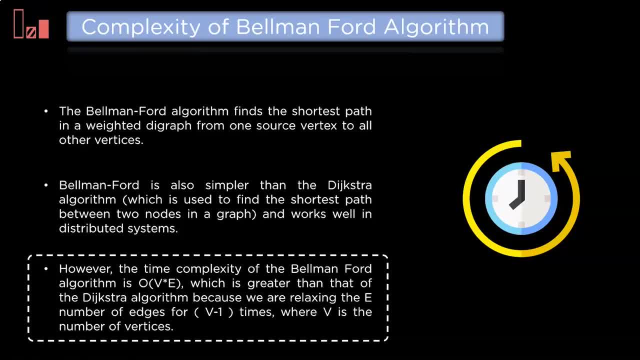 V is the number of vertices. Now, these were the complexities of Bellman-Ford algorithm. Now let us get into practical mode, where we will be executing an example based on Bellman-Ford algorithm. Now on my screen, you can see an example based on Bellman-Ford algorithm. 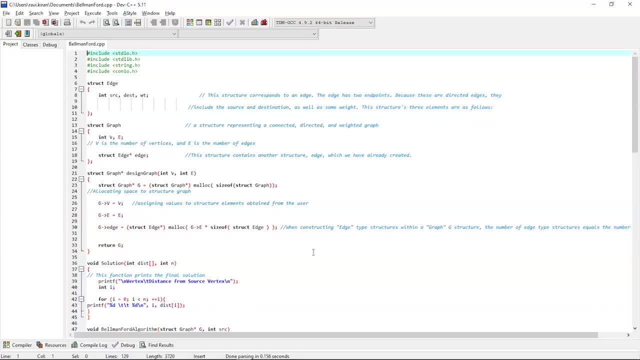 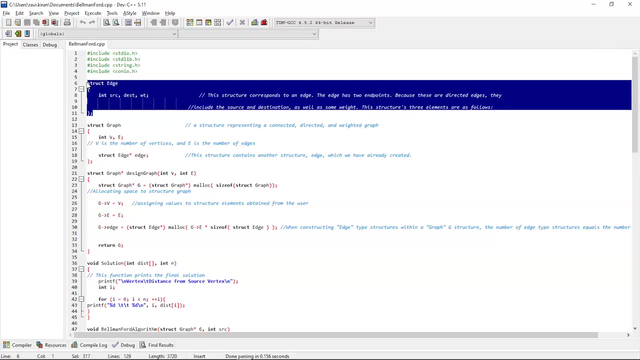 First we finished all the necessary header files, Standard input output, standard library string and all the console input output libraries. Then, using the struct keyword, we created an edge. This structure is equivalent to an edge. There are two endpoints to an edge because these are directed graphs. 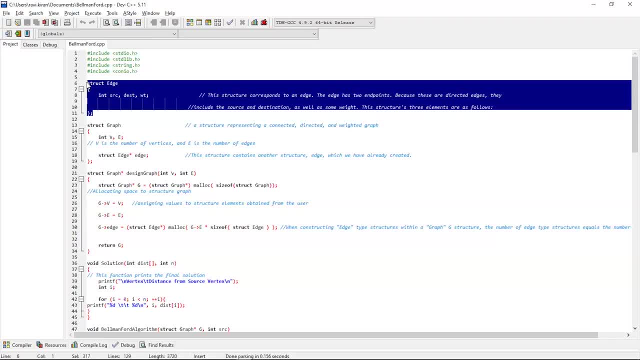 They include the SRC as the source and DESC as destination and some WT as weight. We have created an edge. There are two endpoints to an edge because these are directed graphs. They include the SRC as the source and DESC as destination and some WT as weight. 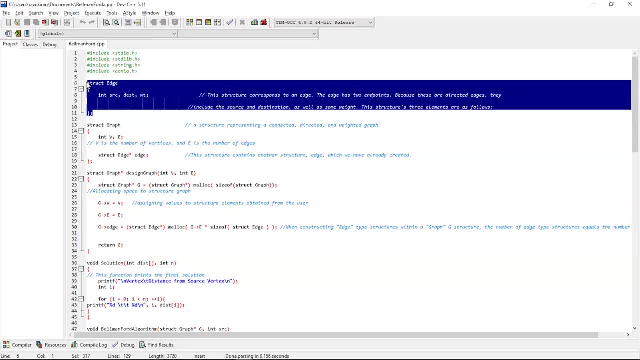 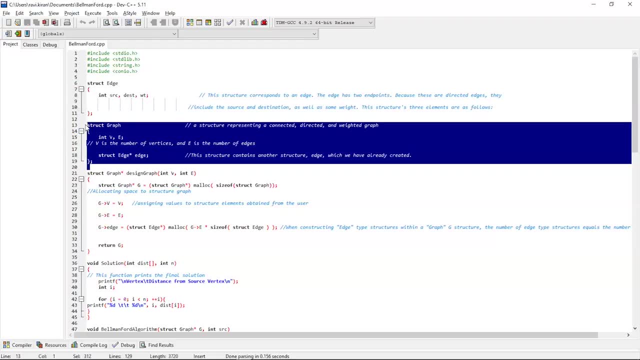 There are two endpoints to an edge because these are directed graphs. We have created an edge Where three components of the structure are as follows. Next, we used the struct keyword to create a graph with two variables, V and E, where V is the number of vertices and E is the number of edges. 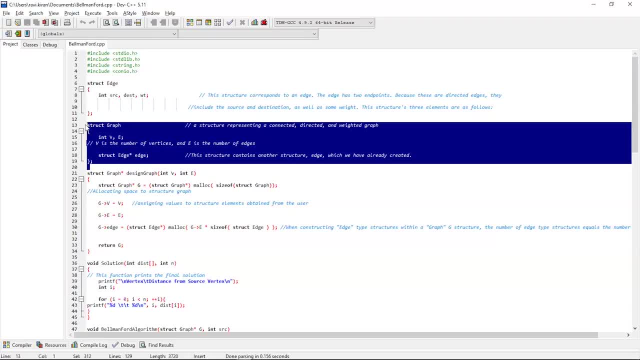 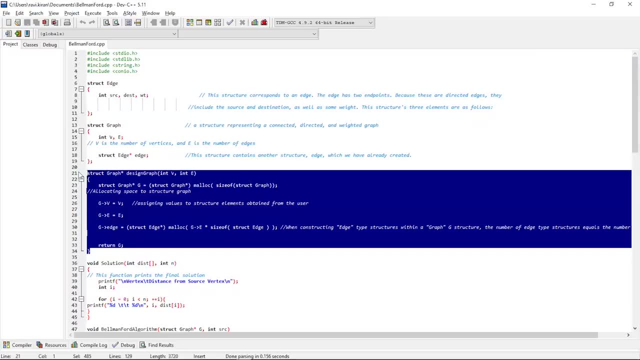 We also made an edge And this structure contains another structure edge which we had previously created. Now we have created a function called Designбоle Graph which contains V and E. using the mallock function, we created a graph. in this function, We assign v and e values to the structure elements obtained. 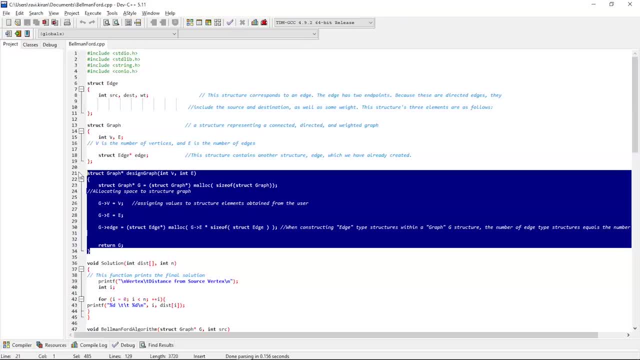 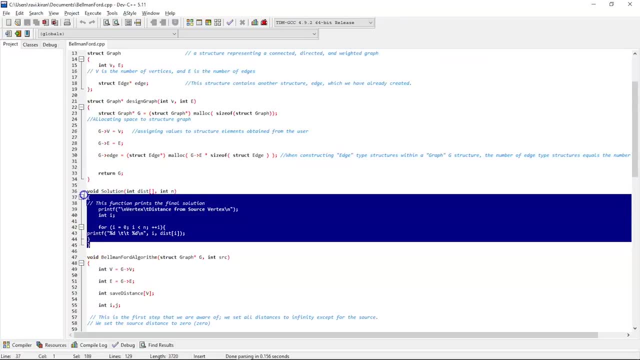 from the user in this graph. Then we make an edge and return the graph. Now we have created a solution which is a function, and this function prints the final solution too. We print the distance from source vertex. For this, we make a loop from 0 to variable n and print the distance. 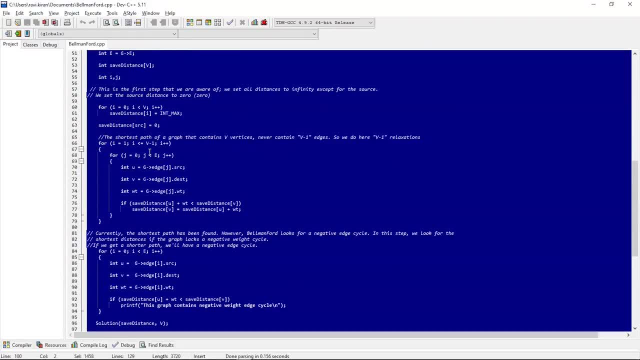 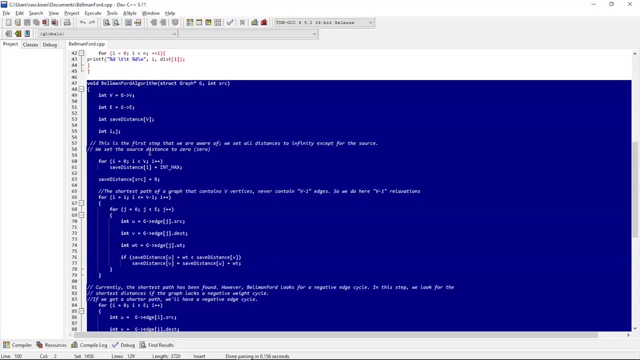 Then we created the Bellman-Ford algorithm function with graph and source variables as parameters and we assign the vertices and edges to the graph again. Finally, we make an array called saveDistanceWithSize as a vertex. After that we declare two counter. 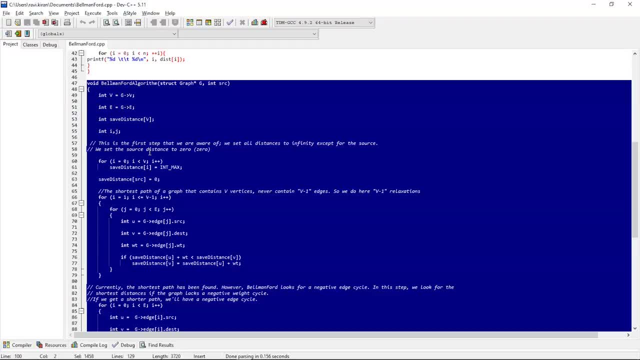 variables i and j. After that, we run a loop from 0 to the number of vertices, and in this loop we set all distances to infinity, except the source, which is set to 0. Now we run a loop from 1 to v minus 1 times, followed by another loop for the edges and 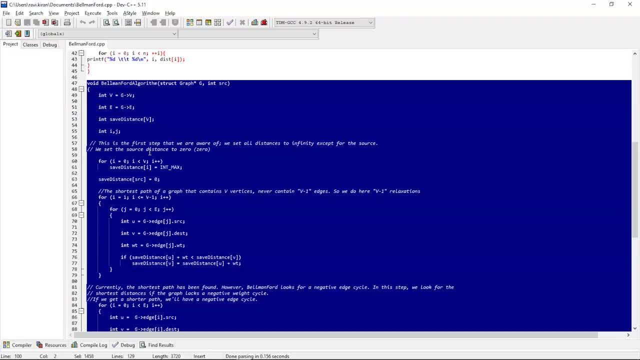 we've declared three variables: u, where we assign the graph source, v, where we assign the graph's destination, and wt, where we assign the graph's weight. Now we have a condition that if the distance of the source node and the weight of the uv edge is less than the distance of the 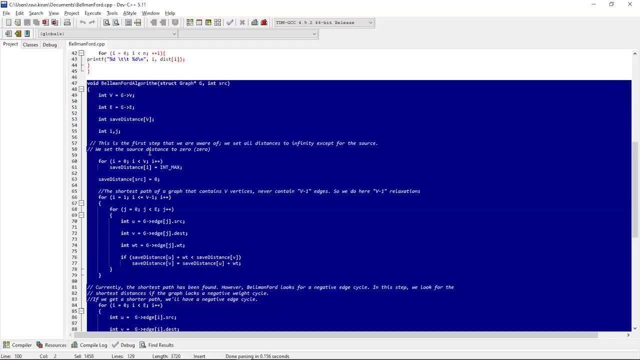 destination node. we update the destination node and we have a condition that if the distance of the source node plus the weight of the uv edge. Now we run a loop from 0 to the graph's edge uv and assign all source, destination and weight of the graph and we have the condition if the 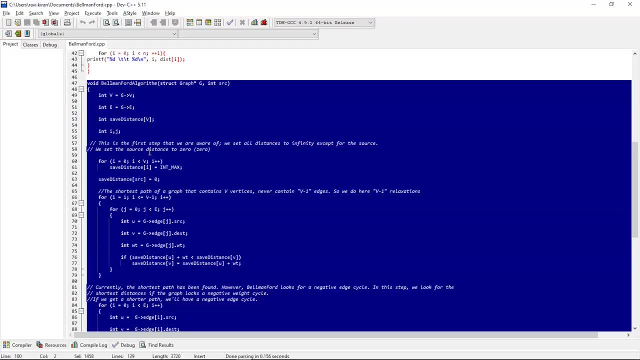 distance of vertex plus the edge of uv is less than the distance of destination vertex, Then we print a graph obtaining a negative edge cycle and call the solution function and return it to v. Finally, we have the main function, in which we have defined three variables as v, e and s. 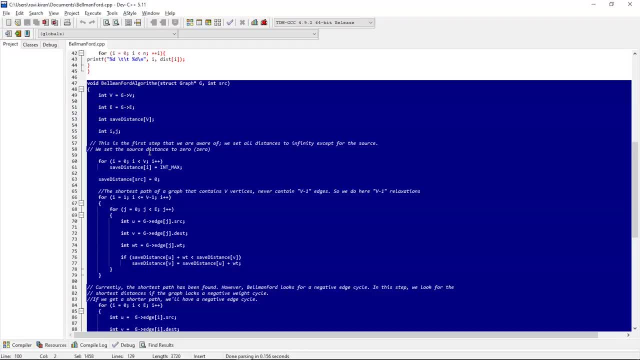 where v is the number of vertices, e is the number of edges and s is the source vertex, And we ask the user to print the number of vertices, edges and source vertex, after which we call the design graph function, which prints the source, destination and weight respectively. 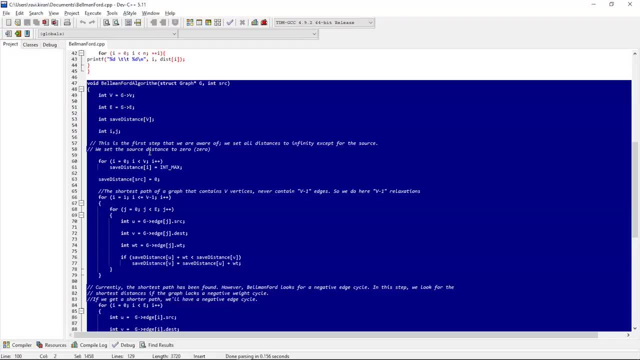 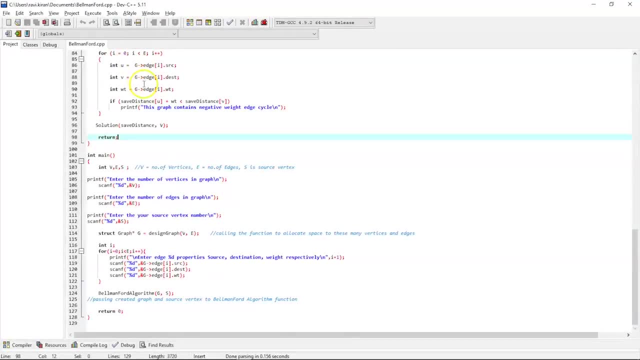 And finally, we call the Bellman-Ford algorithm function to implement the Bellman-Ford algorithm. Now I hope I made myself clear with the code. Let's try to run this code quickly and see the output. So to run this code we might want to press on the execute button. 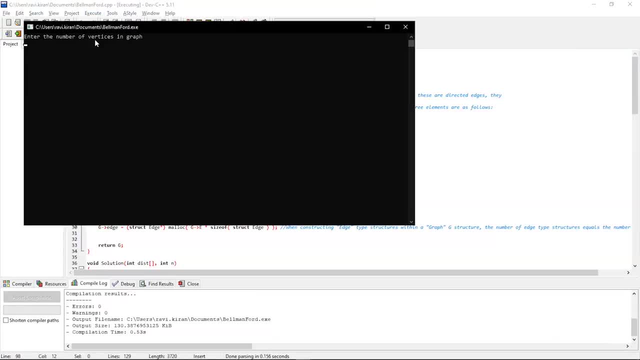 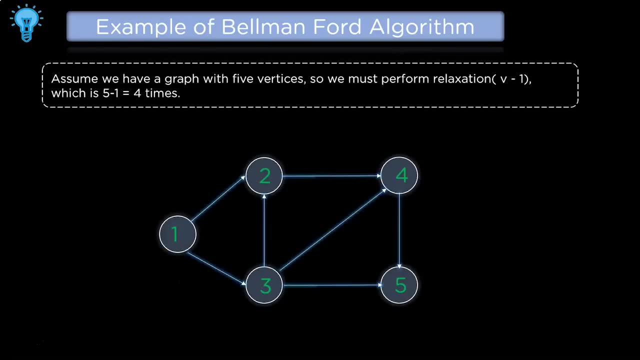 Now let's press the compile and run option. Now you can see that the code got successfully executed and now it is asking for input. Now we will consider the same example that we have seen in the PPT, which is this particular example with five vertices and seven edges and all. the edges are the same. Now we will consider the same example that we have seen in the PPT, which is this particular example with five vertices and seven edges, and all the edges are the same, All the weights which are present in this particular image. 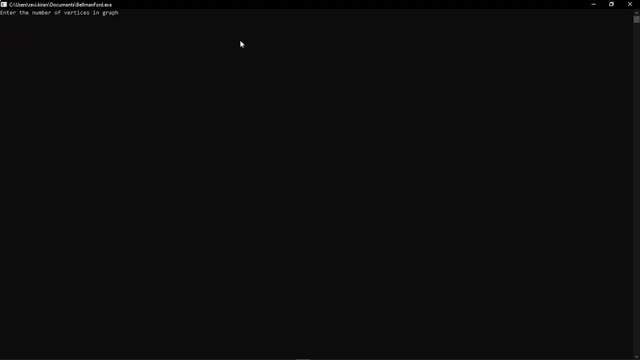 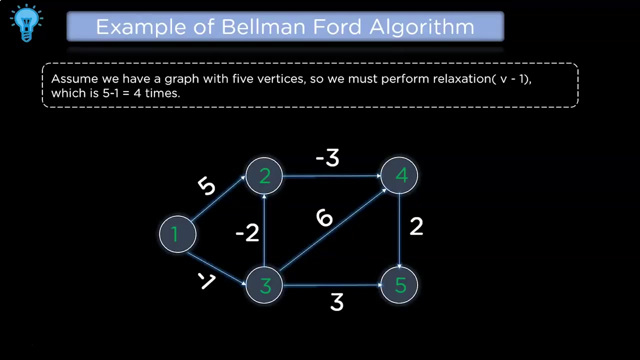 Now let's get back to the output window and try to provide the inputs. So enter the number of vertices in graph- So we have five vertices in this particular graph. As you can see, we have five vertices- and enter the number of edges in the graph. 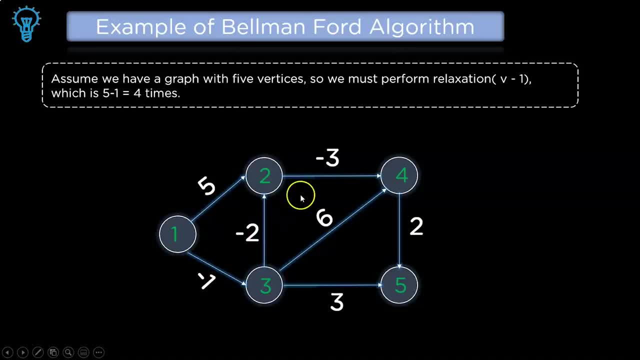 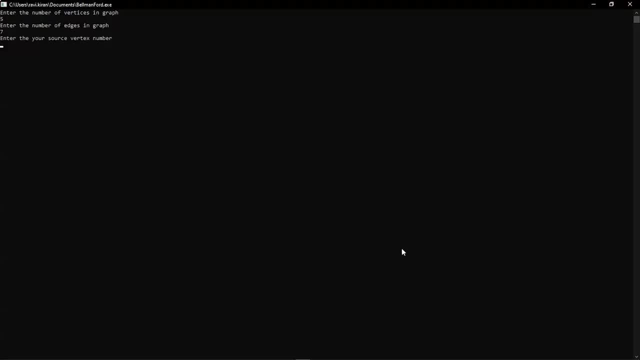 So let's count the edges. So 1,, 2,, 3,, 4,, 5,, 6 and 7.. So we have seven edges in the graph. Now enter the source vertex number. So the source vertex number is one, So 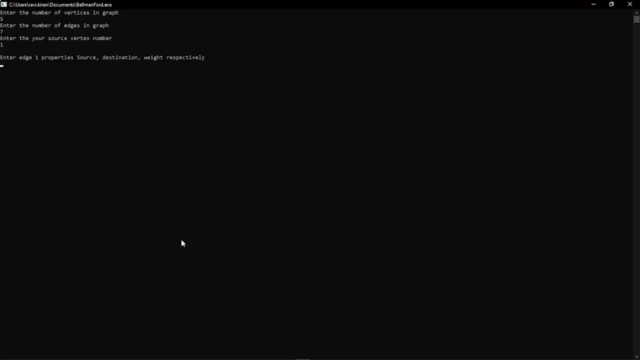 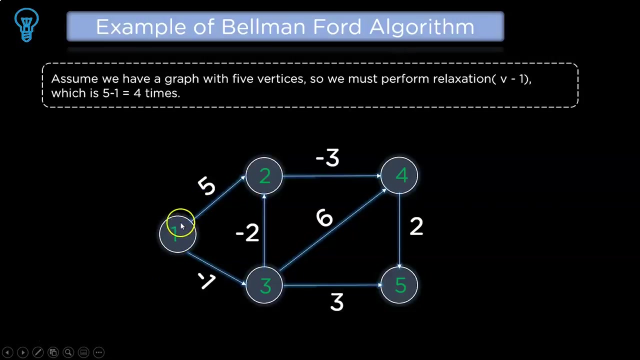 let us provide one Now. enter the edge1 properties. So we have to enter the source of the edge one, its destination and its weight respectively. So here we have the first edge, that is 1 to 2.. So the source is one and the destination is two and the weight is five. So we have to. 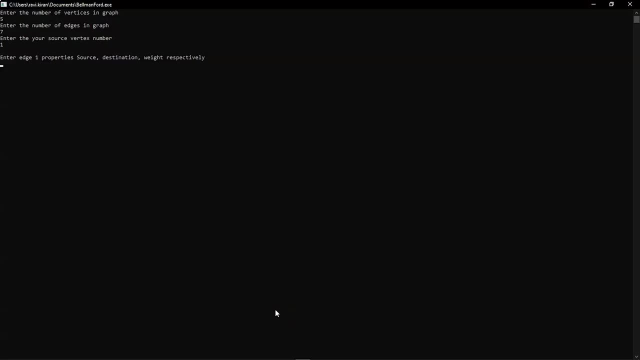 enter 1,, 2 and 5 and so on. So the source is 1,, destination is 2 and weight is 5.. Now it will ask for the next edge, that is edge 2.. Let us finish all the edges from vertex 1.. 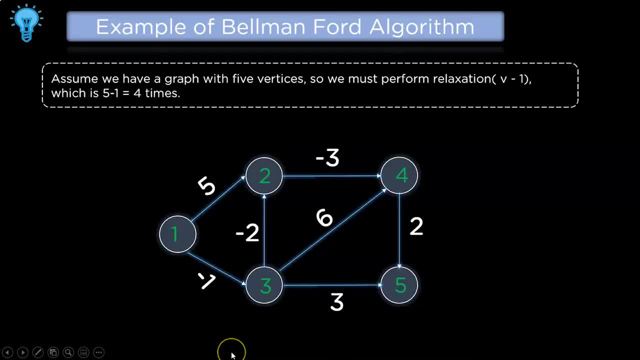 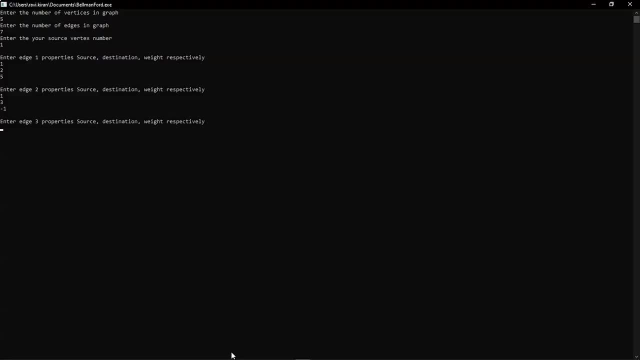 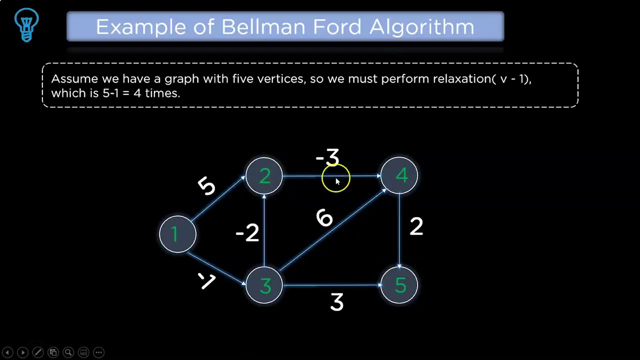 So again, we will provide the source as 1 and destination as 3.. So the weight is minus 1.. Now enter the edge 3 properties. Now let us go to the vertex 2.. So from vertex 2 we have just one edge which is going towards 4.. 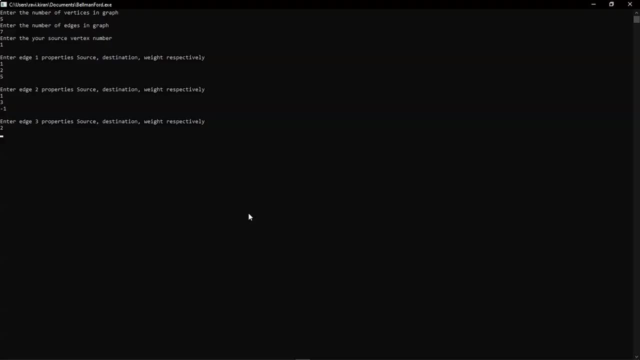 Let us enter the data: Source is 2, destination is 4 and weight is minus 3.. So let us go to the next vertex, that is 3.. So from 3 we have 3 edges. So let us enter the data 3 and the first destination is 2, with weight minus 2.. 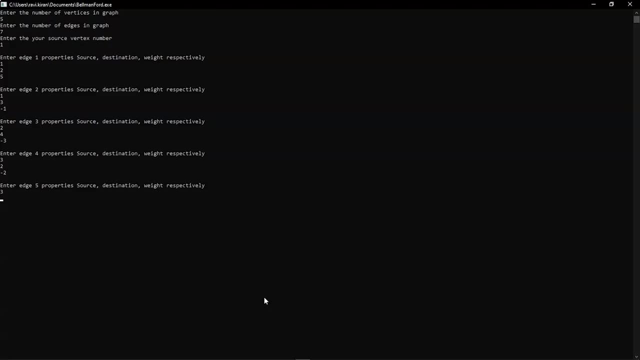 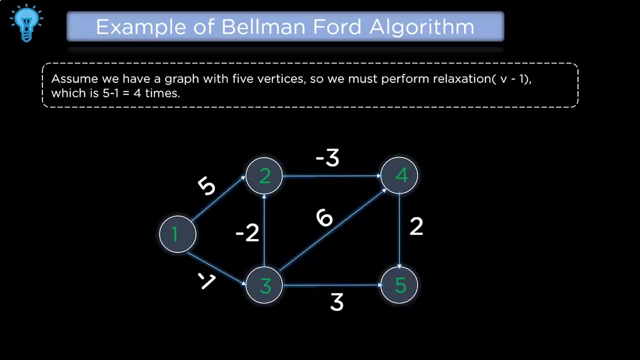 Now the source will be 3 again. This time it is going towards 4 with weight 6.. Another last edge, that is from source 3 to destination 5 with weight 3.. Now the 7th edge, that is 4 to 5.. 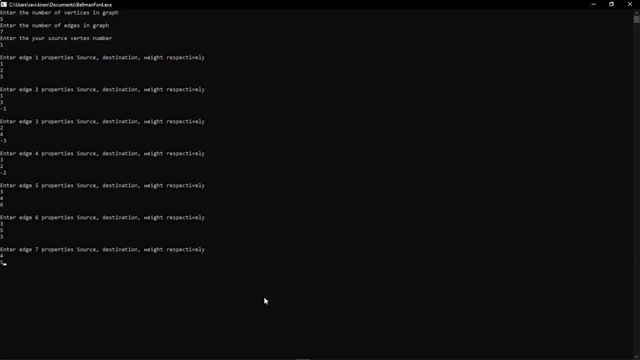 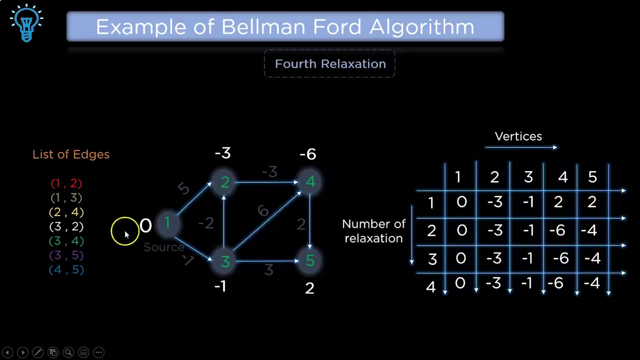 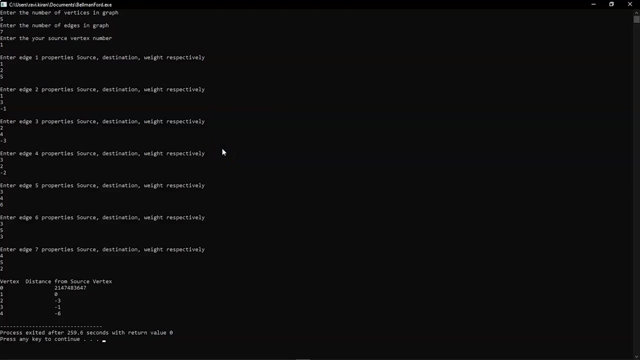 So the source is 4, destination is 5 and the weight is 2.. So let us enter and we will have our answer. So the vertex- distance from the source vertex- is here. you can see the answers. So from 1 we have 0 and from 2 we have minus 3- that is here- and from 3 we have minus 1, which. 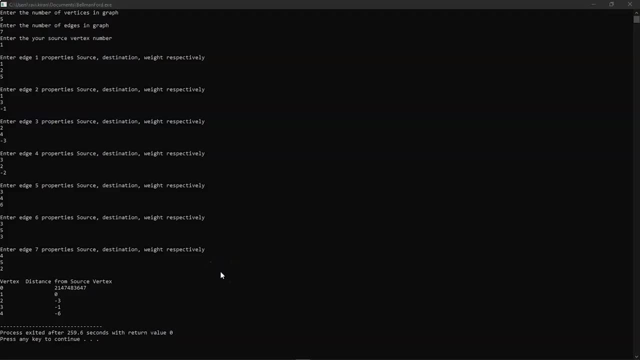 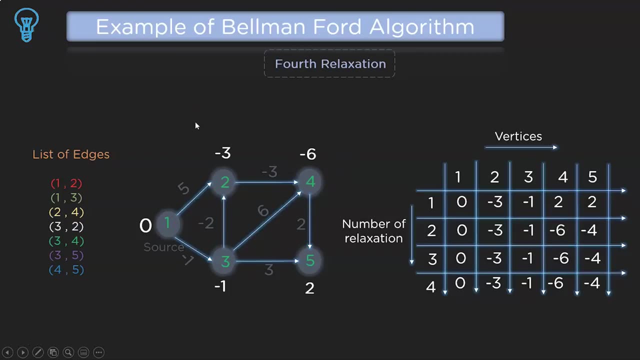 is over here, and from 4 we have minus 6, which is over here. This is how you get the result for Bellman-Ford's algorithm and this is how you implement it. So with that, we have come to an end of this session on Bellman-Ford's algorithm. and if